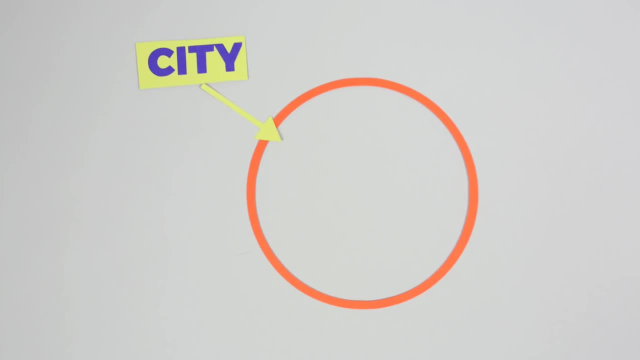 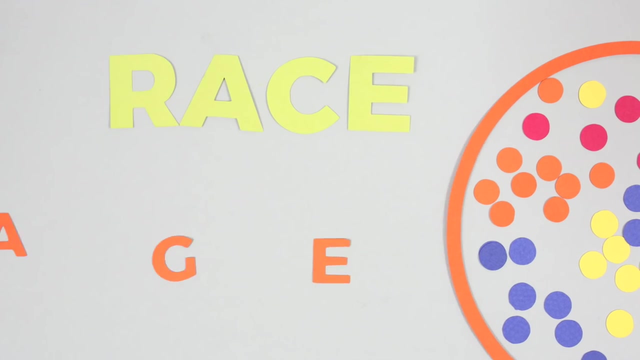 Okay, so this is a city. Here are all the people living in it, People of all different colors, ages, wealths and incomes, Except they don't all live together in the same place. They're separated into different parts of the city by what color they are, what language they speak and how much money they have. 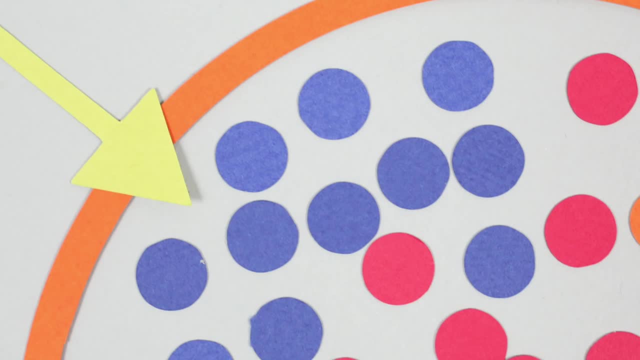 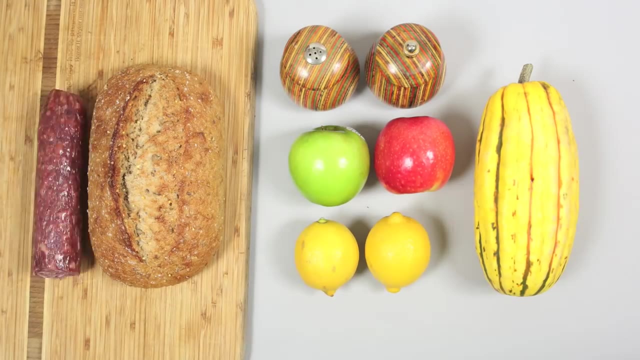 And those different parts of the city look quite different. The parts that are whiter and wealthier tend to have green spaces, grocery stores with nutritious organic food and, of course, somebody to buy it, and are often far away from pollution-emitting freeways. 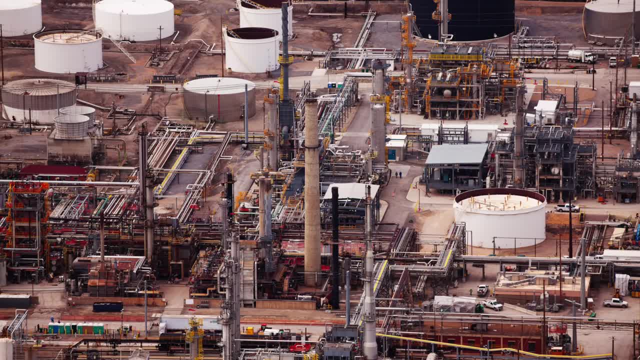 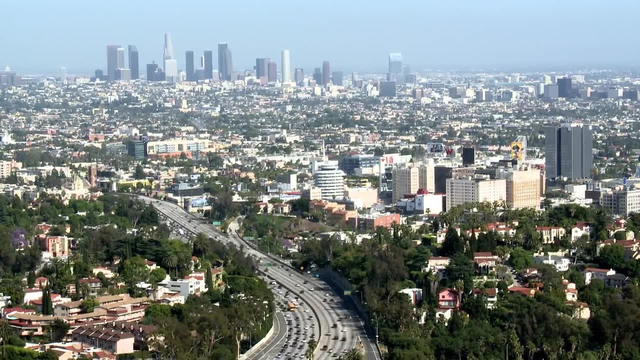 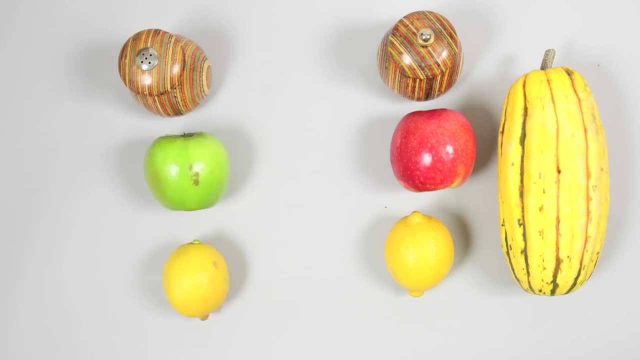 The parts that are poorer and more diverse tend to have industrial sites, heavy-duty, diesel-polluted ports and highways and hazardous waste- All things that the city relies on to run properly but that heavily pollute the air and water. And even if they had those grocery stores with nutritious organic food, 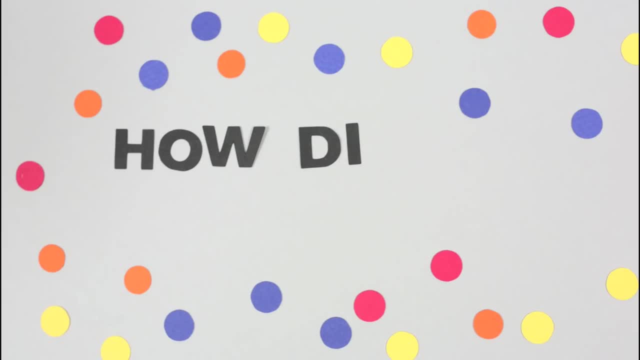 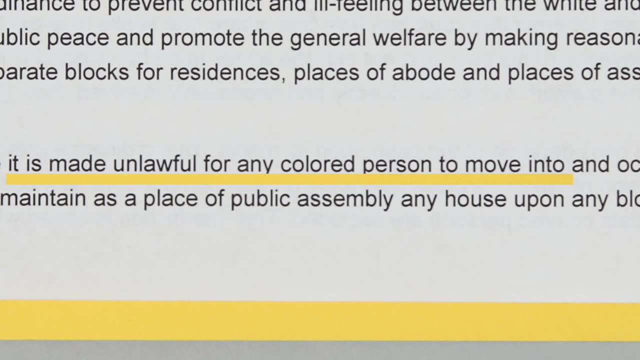 most of the time, most residents there couldn't afford it anyway. How did this happen? Well, this segregation can be traced back to race-based zoning and housing policies, But it wasn't always as deliberate as plain old racism. Some separations can simply be traced to poor land use planning. 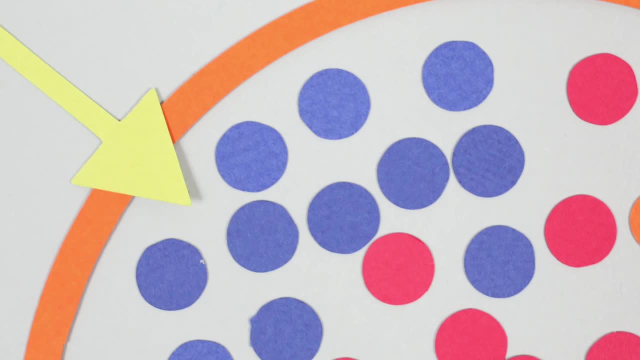 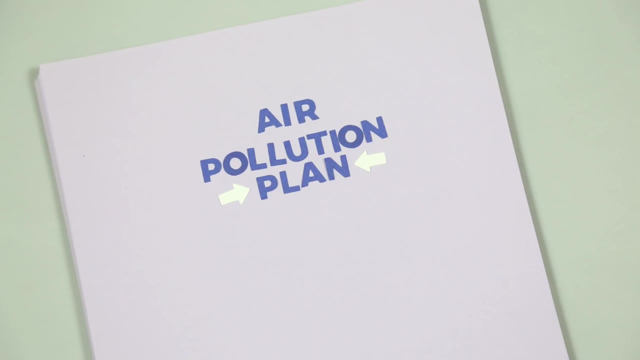 And, as a result, these residents of the same city live very different lives. Say, the city realizes it has an emissions problem, It comes up with a plan to reduce air pollution. plant more trees to suck up the carbon, start a cap-and-trade program. 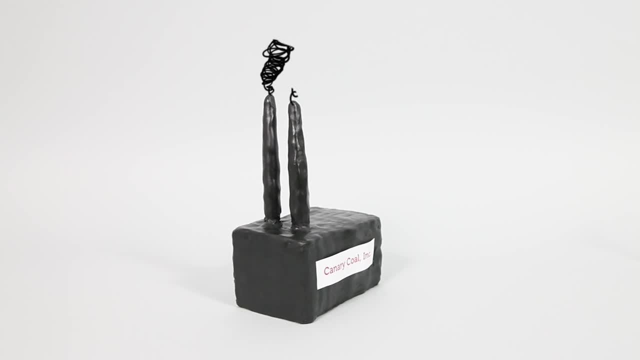 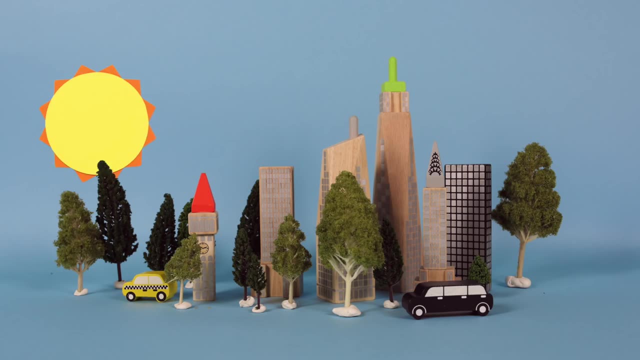 But those trees get planted in the neighborhoods that are already green And the factories that are spewing toxins into the air just buy more carbon offsets and keep spewing their toxins. The benefits of these programs are enjoyed by the communities that are already doing just fine. 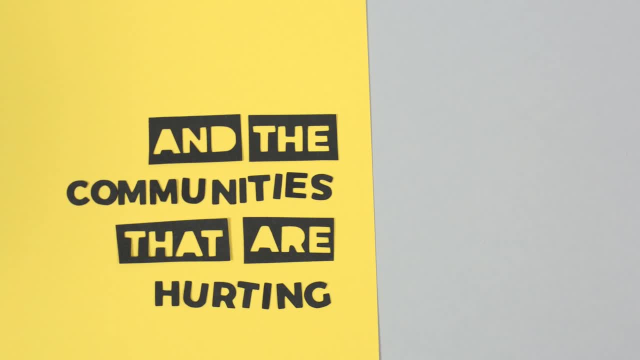 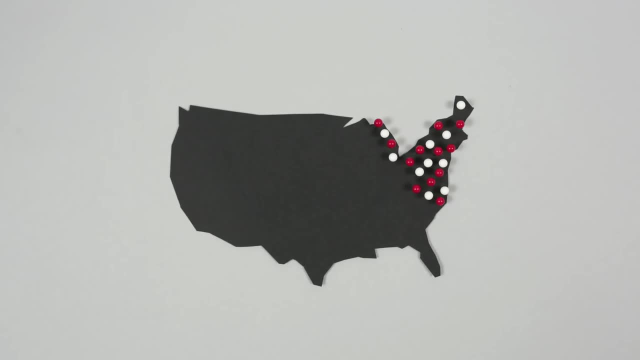 And the communities that were hurting most from all that air pollution. Well, they're still hurting. This isn't just an imaginary city. This is the story of real cities all across the US Where people might live in the very same area code. 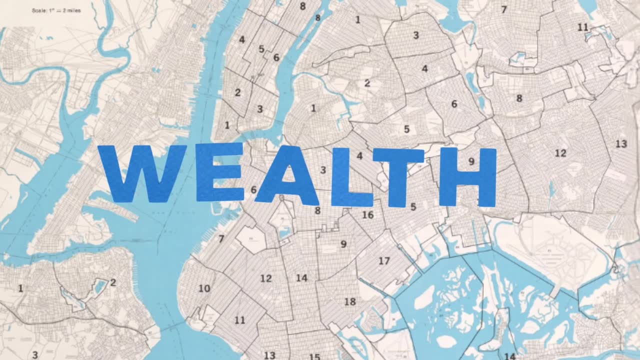 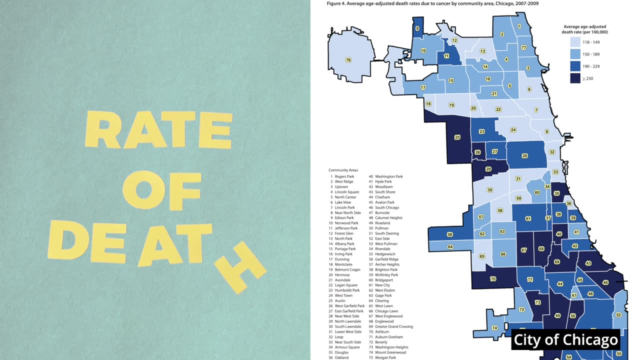 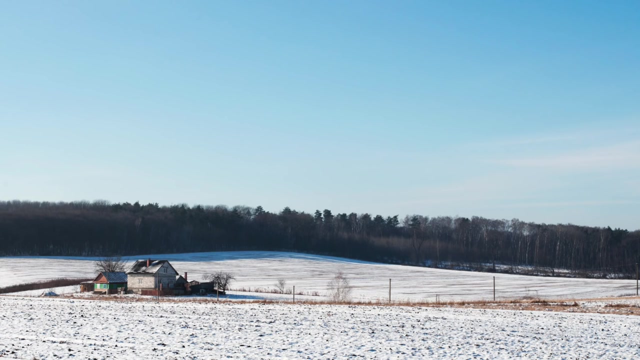 but their race, ethnicity or wealth and income bracket causes them to experience wildly different quality of air, water and life. In fact, it can even mean that they also experience different deaths. That's how serious this stuff is. This kind of inequity expands far beyond cities too.